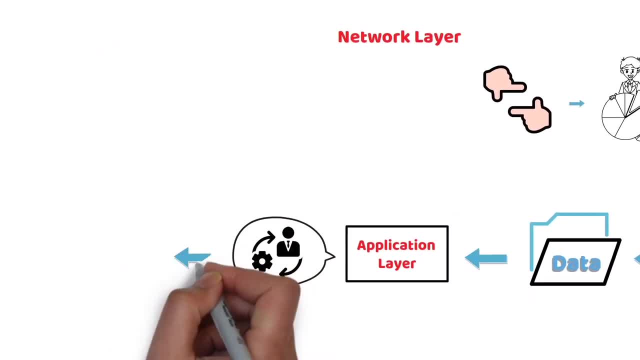 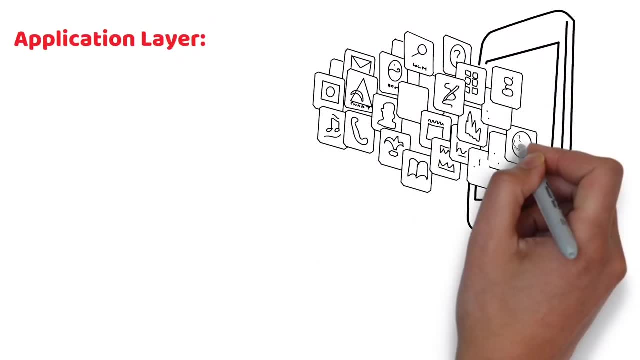 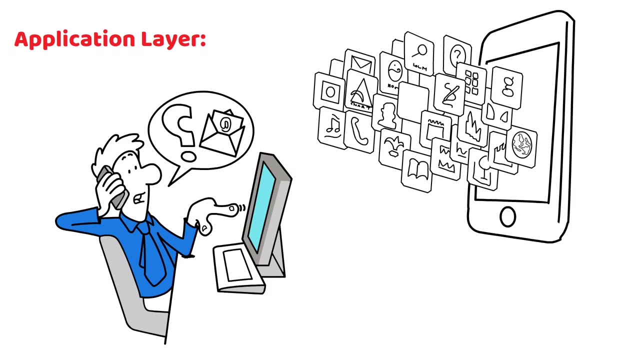 The Application Layer feeds the human-readable data to the email software that will allow your friend to read your email. Application Layer. The Application Layer is where the user interacts with a software application, so it is closest to the end user. This layer interacts with the application communicating with the network. 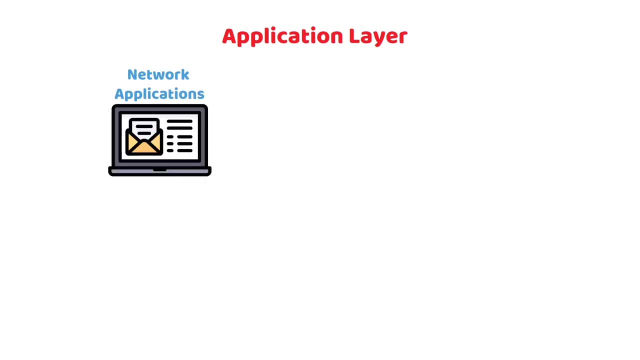 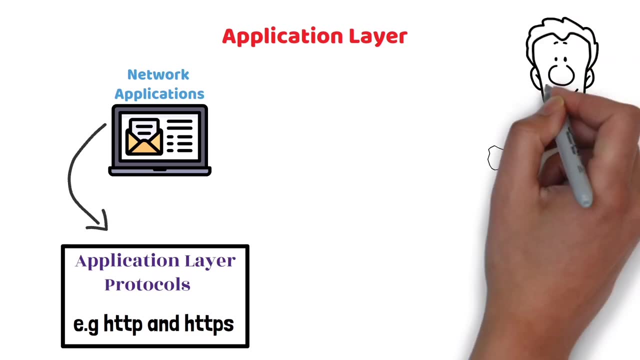 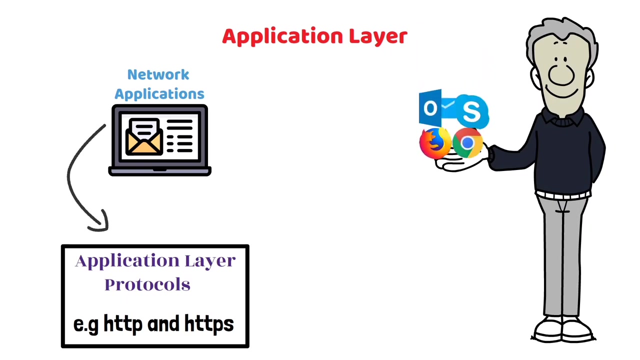 Application Layer. Application Layer is used by network applications which rely on Application Layer protocols like HTTP and HTTPS to function. The applications that use these protocols are browsers, Firefox, Google Chrome, Outlook, Skype, etc. There are many Application Layer protocols that enable functions at this layer. 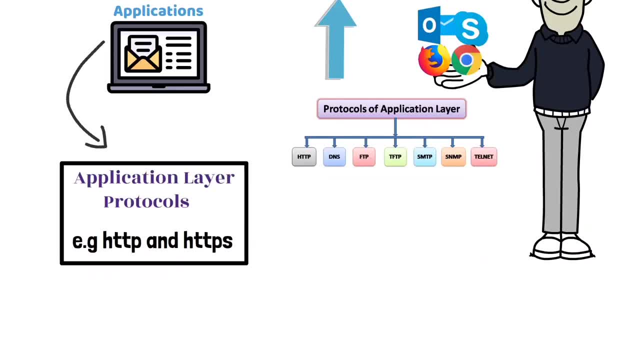 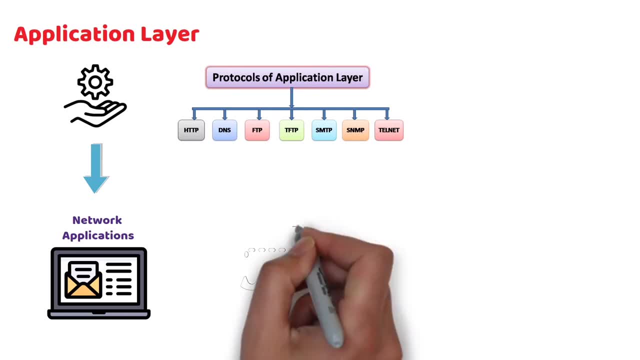 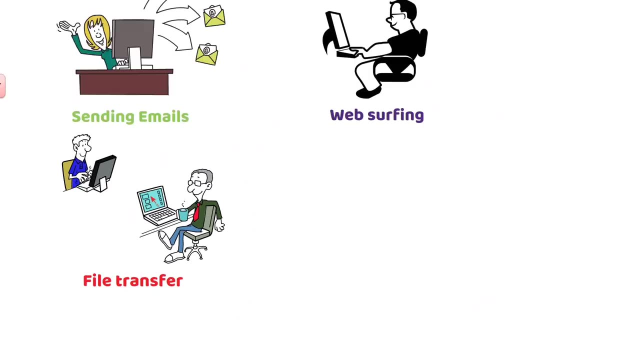 All these protocols collectively called Application Layer. Application Layer provides services for network applications. With the help of these protocols, users are able to perform activities like sending emails, file transfer, web surfing, etc. File transfer is done with the help of FTP protocols. 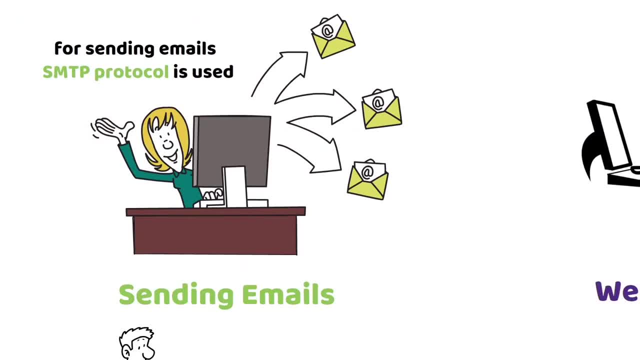 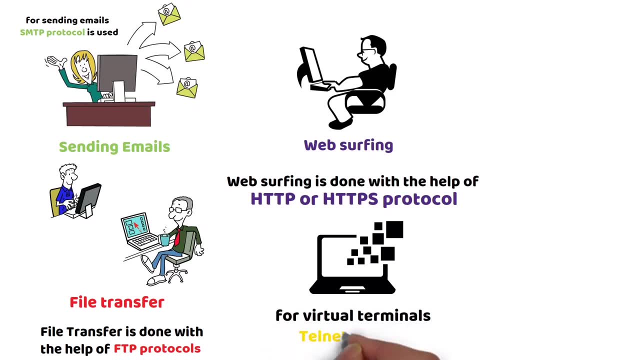 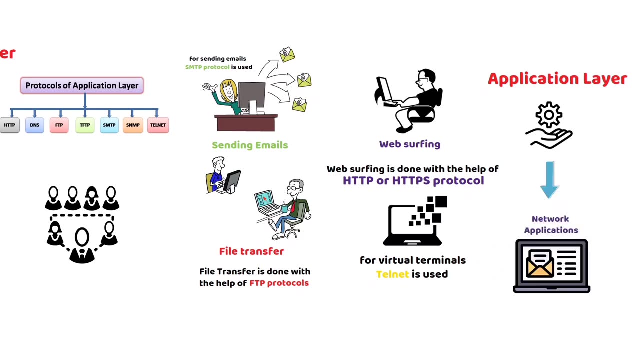 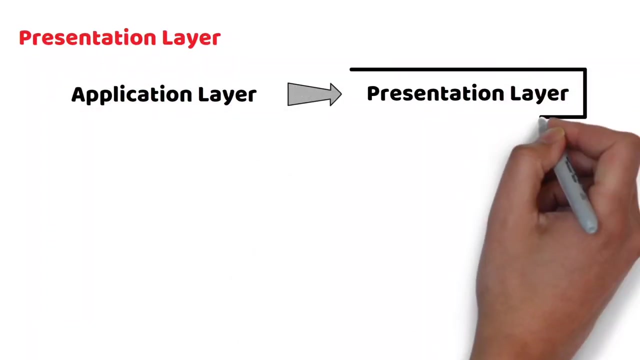 For sending emails, SMTP protocol is used. Web surfing is done with the help of HTTP or HTTPS protocol, And for virtual terminals, Telnet is used. Application Layer provides services for network applications. Presentation Layer. Next to Application Layer is the Presentation Layer. 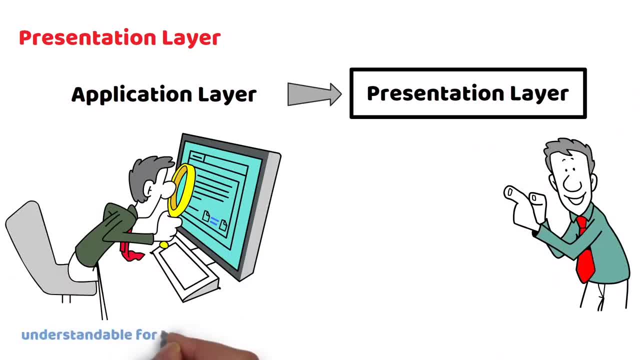 This layer is responsible for ensuring that the data is understandable for the end system or useful for later stages. It translates or formats data based on the application's syntax or semantics. It also manages any encryption or data transfer. It also manages any encryption or data transfer. 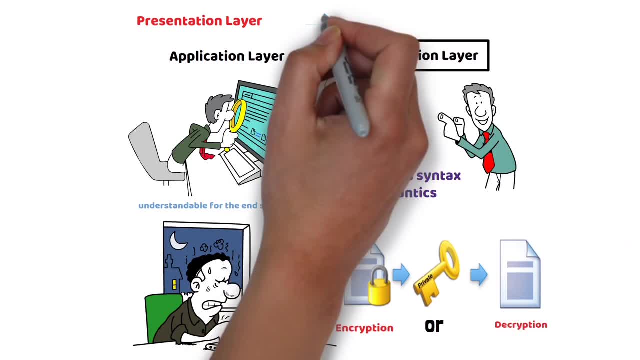 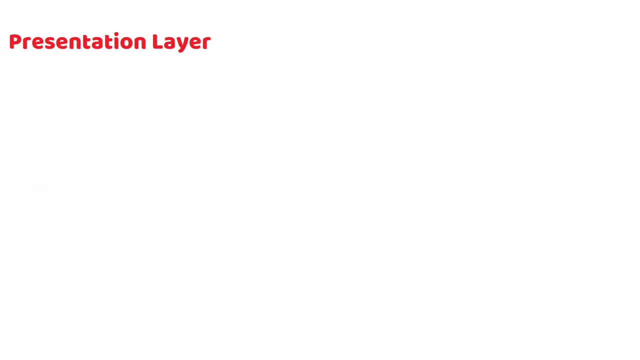 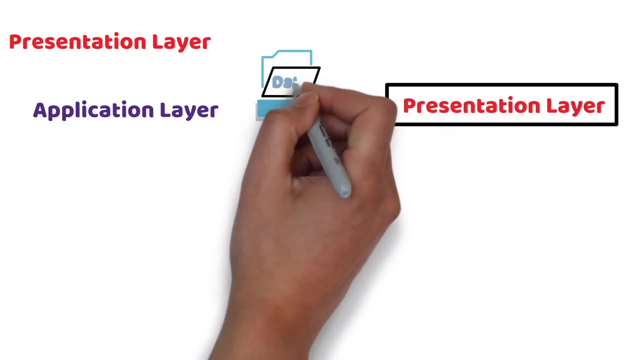 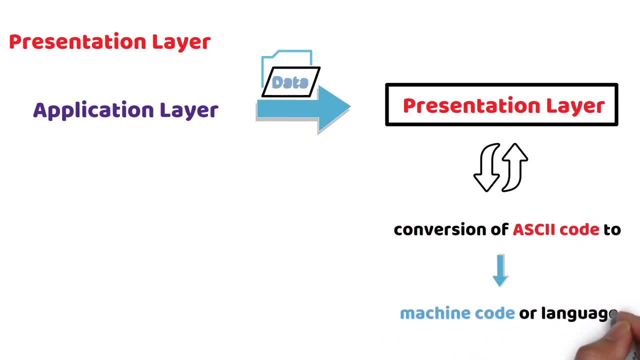 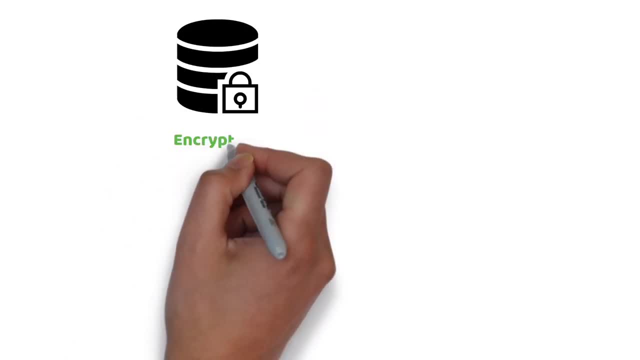 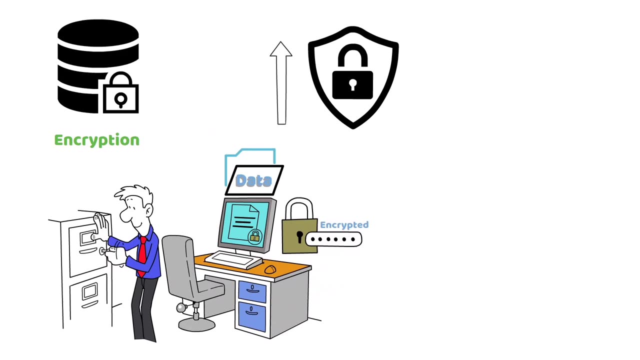 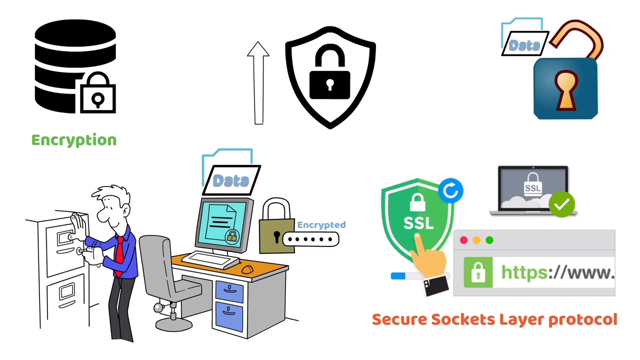 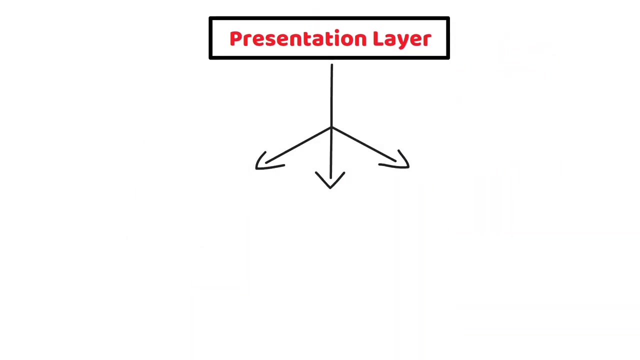 currently out of service. This recalled Encryption enhances the security of sensitive data. at sender side, Data is encrypted. at the receiver side, Data is decrypted as protocols, or SecureSocket's layer protocol is used in presentation layer for encryption and decryption. So presentation layer performs three basic functions: transmission, compression and 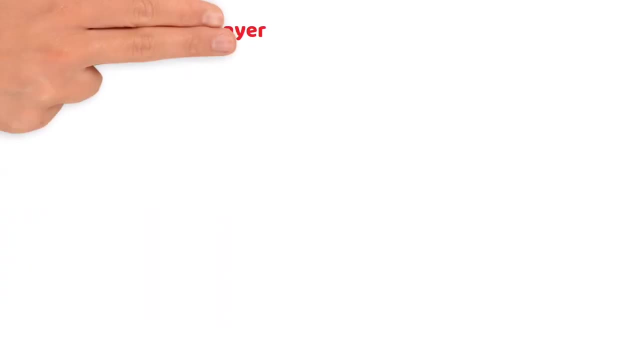 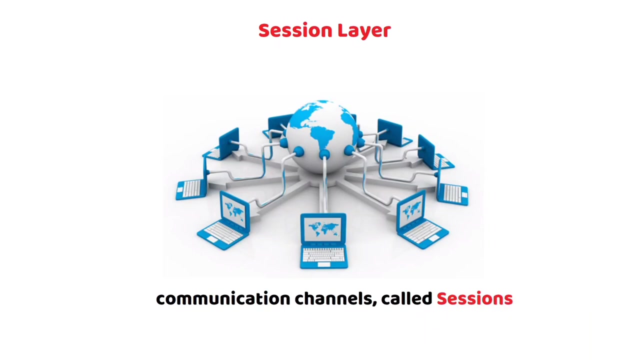 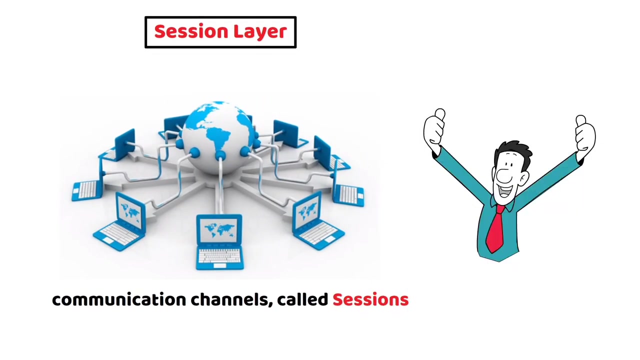 encryption-decryption Session layer. The session layer will create communication channels, called sessions, between different devices. This layer is responsible for opening those sessions and ensuring that they're functional during data transfer. In other words, the session layer is responsible for establishing, managing and terminating. 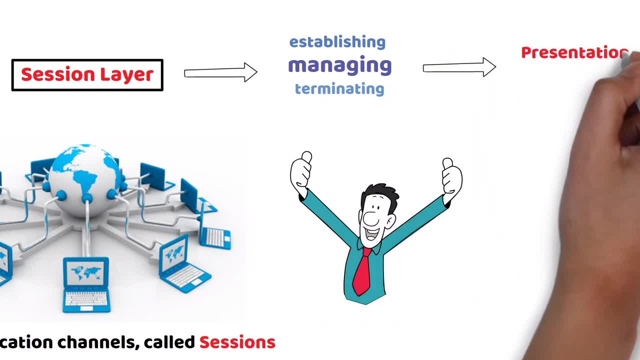 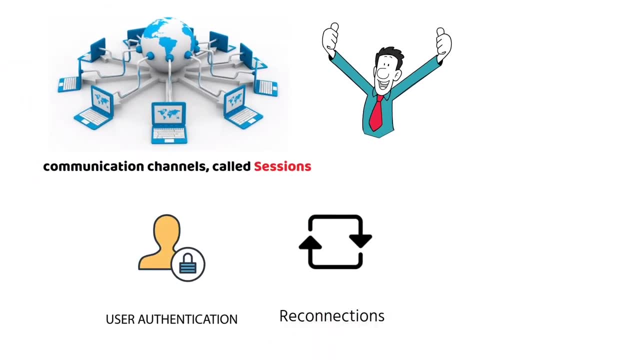 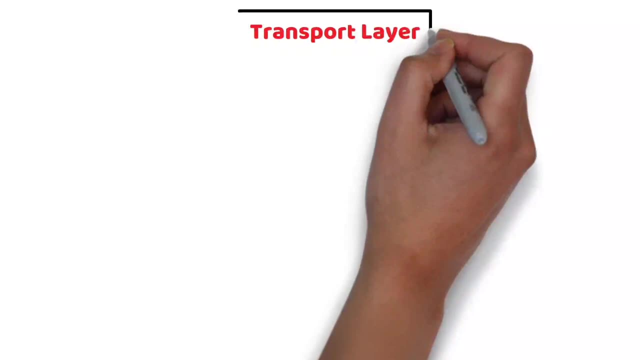 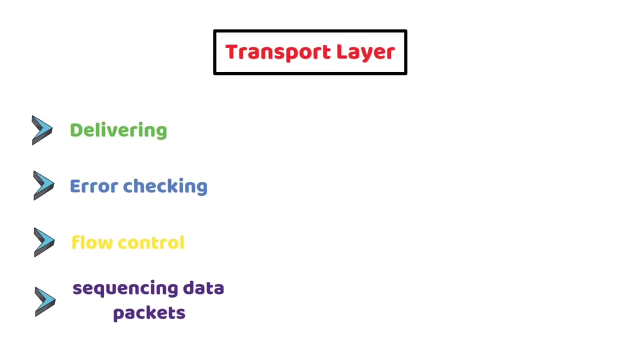 communication sessions with the lower layers, with the presentation and communication layer. It is also responsible for authentication and reconnection And it can set checkpoints during a data transfer. Transport layer: The transport layer is responsible for delivering, error checking, flow control and sequencing data packets. 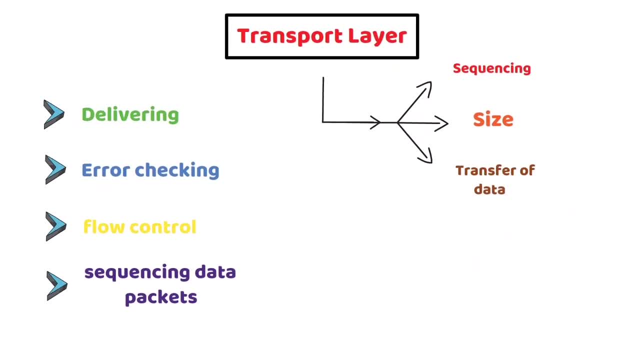 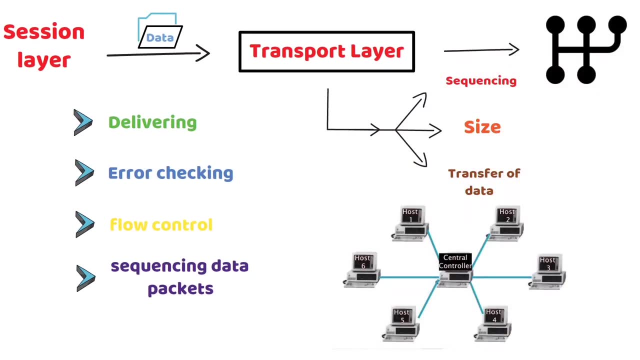 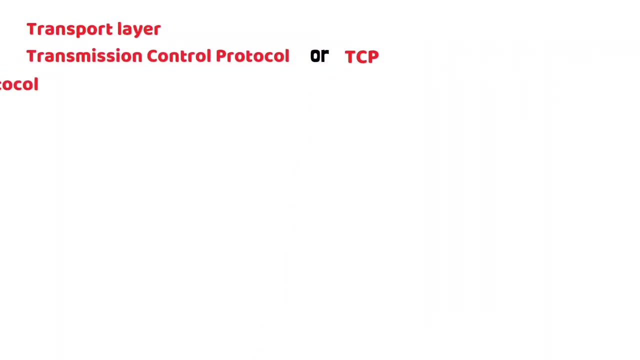 It regulates the sequencing, size and transfer of data between systems and hosts. It gets the data from the session layer and breaks it into transportable segments. Protocol from transport layer is responsible for monitoring, monitoring, monitoring and tracking. the data Transport layer is responsible for monitoring, tracking, monitoring and testing. why the 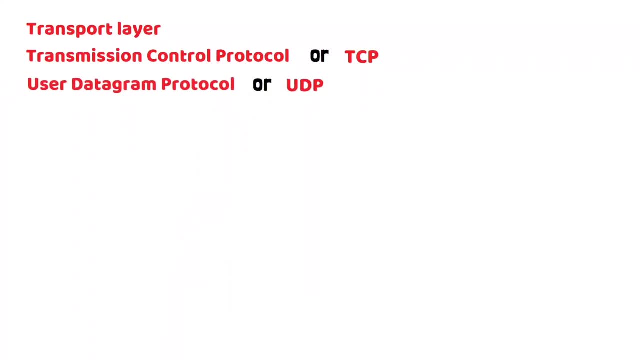 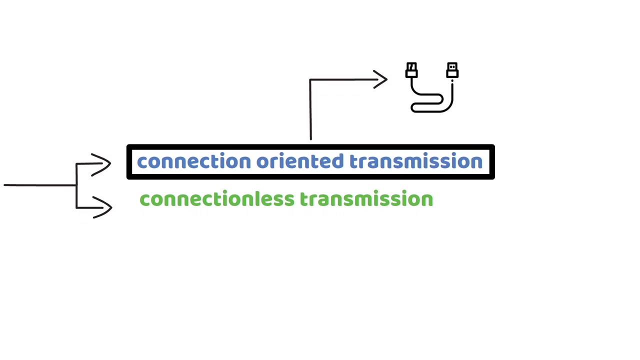 data is being sent and ignoring and running Transport layer Or transmission control protocol, or TPT, and user datagram protocol or UDP. Transport layer performs two types of services: connection oriented transmission and connectionless transmission. Connection oriented transmission is done via wire connection. 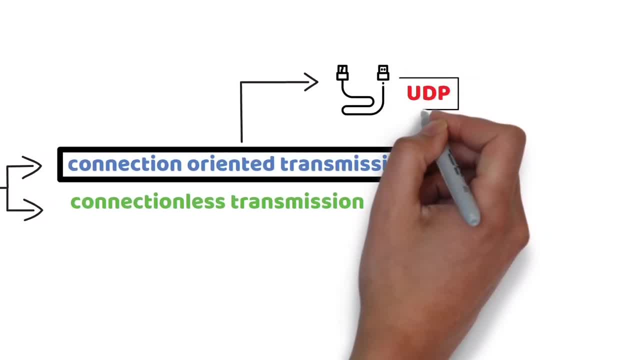 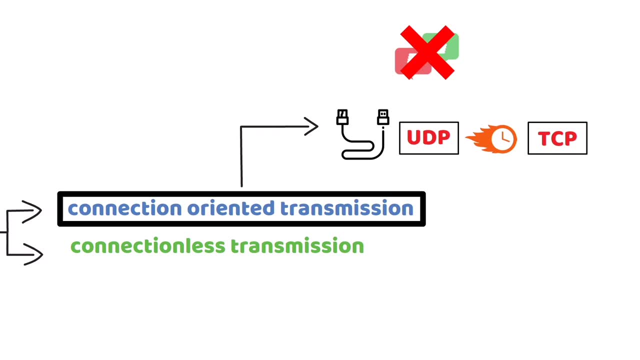 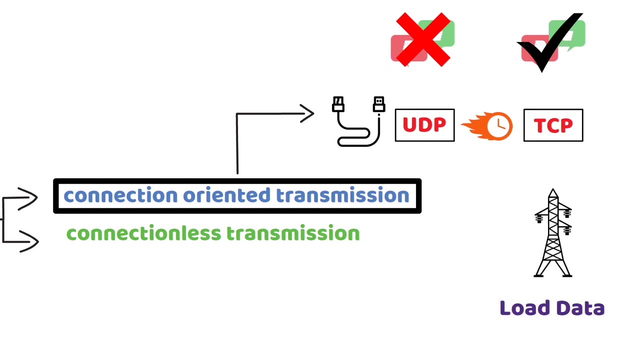 This transmission is done by UDP. UDP is faster than TCP because it does not provide any feedback whether data is been sent or received, whether data has really transferred, whereas TCP provides a feedback. Therefore, load data can be retransmitted in TCP. 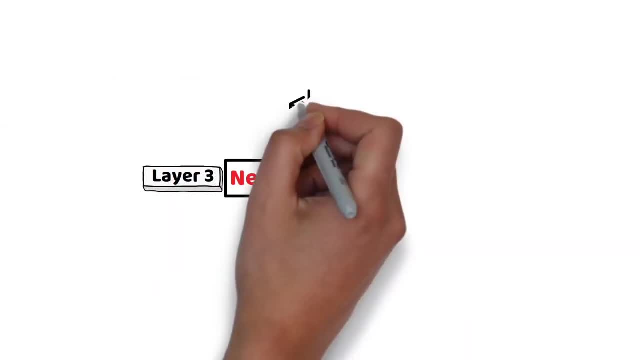 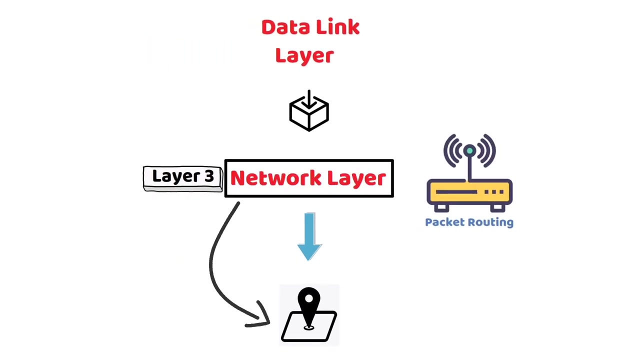 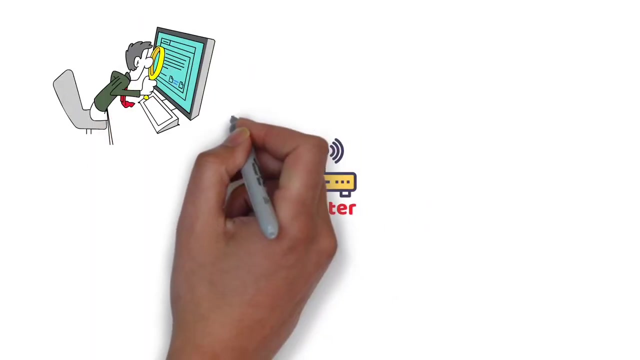 Layer 3 – Network Layer. The network layer receives frames from the data link layer and delivers them to the intended destination based on the addresses inside the frame. It also handles packet routing. The network layer locates destinations using logical addresses, like the IP. Routers are a crucial component at this layer, as they route information to where it needs. 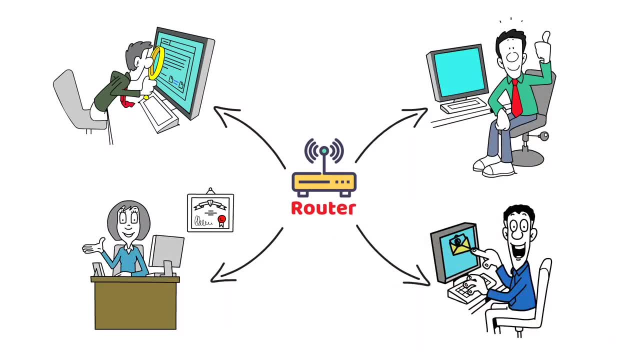 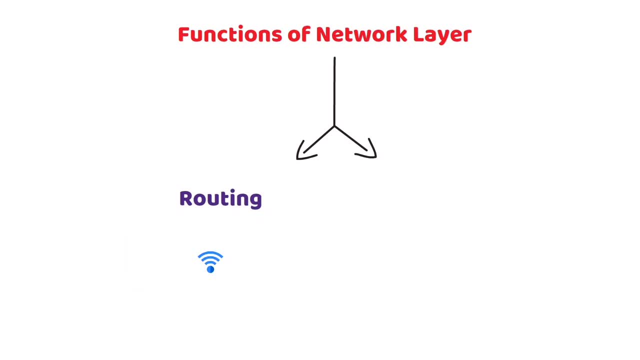 to go between different networks. The main functions of the network layer are: Routing – The network layer protocols determine which routes from source to destination. Logical Addressing – The network layer defines an addressing scheme for each network layer. However, the network layer controls the address addresses that will be sent to the Wrong address. 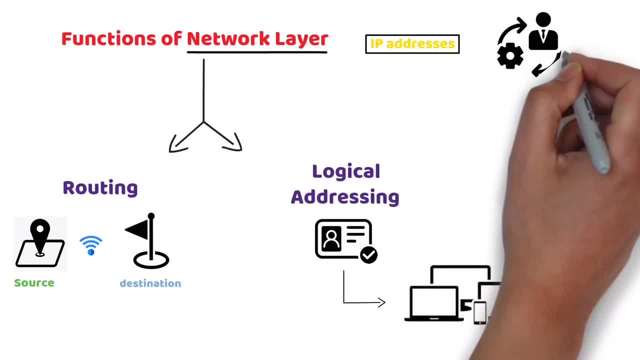 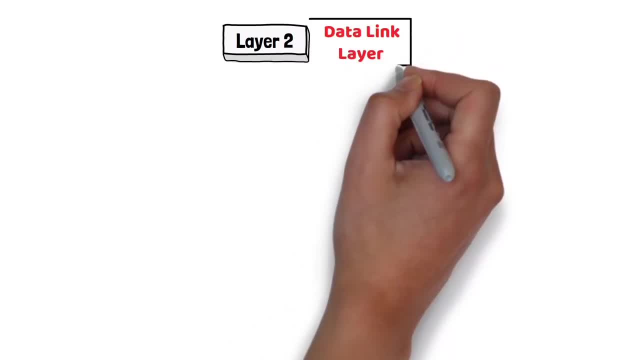 and the address addresses to be sent to the wrong address. The network layer controls how the address addresses are placed from the sender and receiver in the header Layer 2 – Data Link Layer. The data link layer directs any errors that may have occurred at the physical layer. 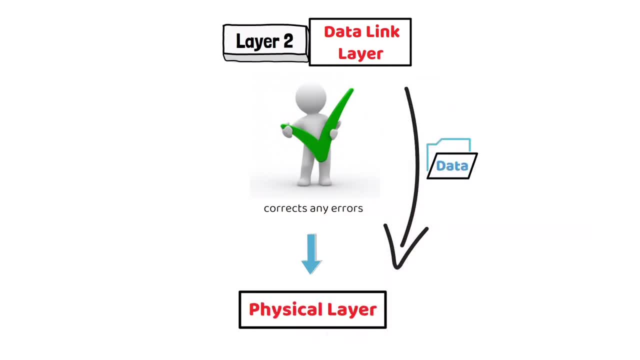 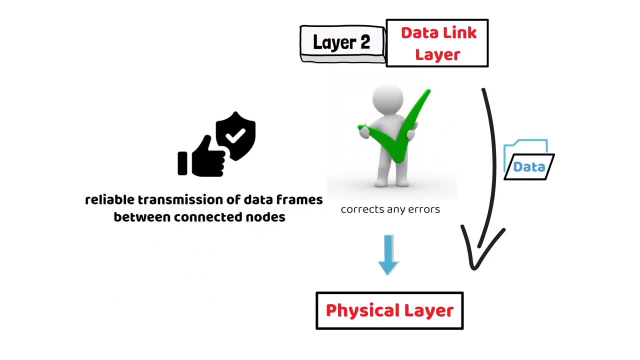 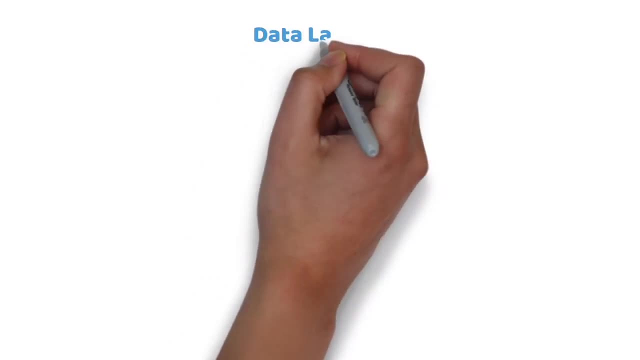 It ensures that any data transfer is error-free between nodes over the physical layer. It is responsible for reliable transmission of data frames between connected nodes. The data is packaged into frames here and transferred node to node. The data layer has the following sub-layers: 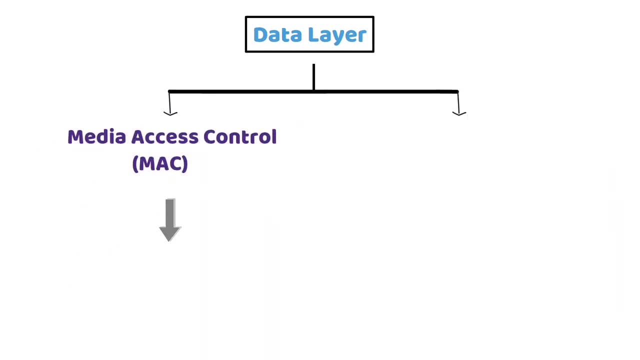 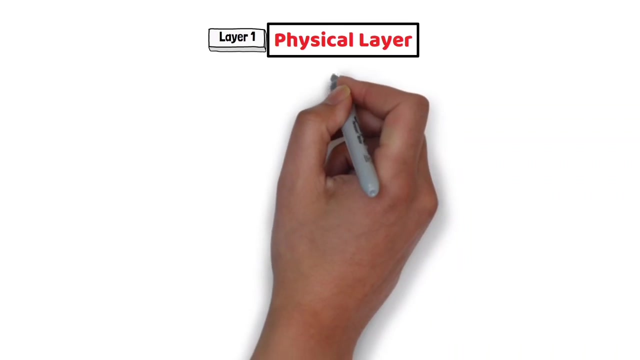 Media Access Control: The MAC address layer is responsible for flow control and multiplexing devices' transmissions over the network. Logical Link Control: The LLC layer provides error control and flow control over the physical medium and identifies line protocols. Layer 1 – Physical Layer: The physical layer is responsible for transmitting. 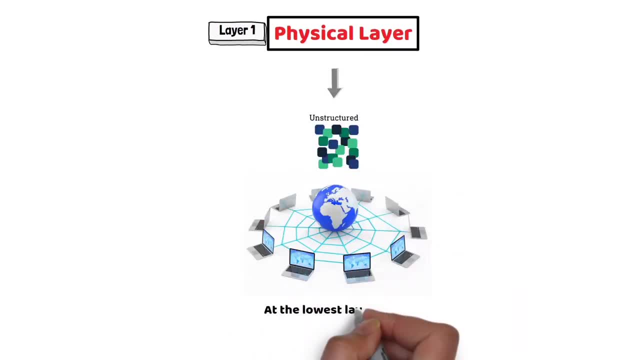 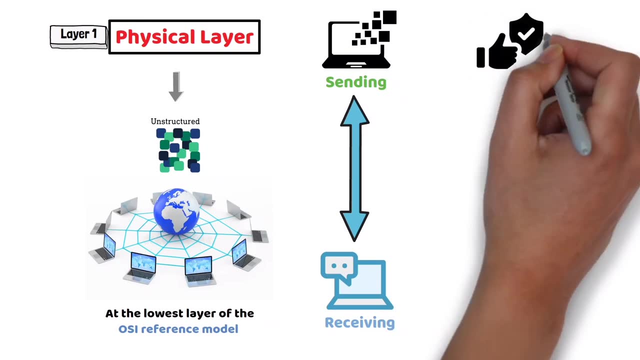 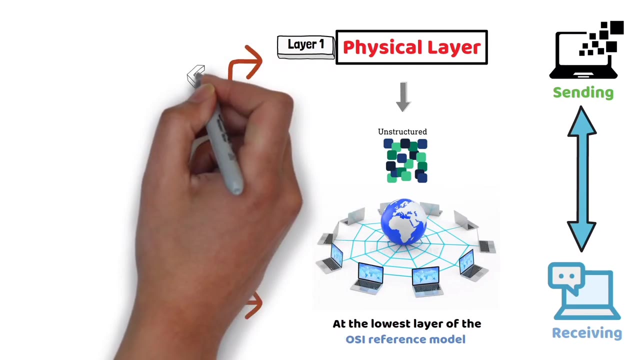 unstructured data bits across the network at the lowest layer of the OSI reference model between the physical layers of the sending and receiving devices. In other words, it takes care of the transmission of raw bit streams. The physical layer may include physical resources like cables, modems, network adapters and hubs etc.